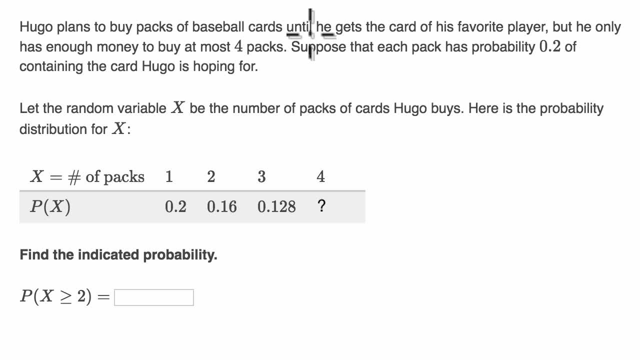 Hugo plans to buy packs of baseball cards until he gets the card of his favorite player, But he only has enough money to buy at most four packs. Suppose that each pack has probability 0.2 of containing the card Hugo is hoping for. Let the random variable x be the number. 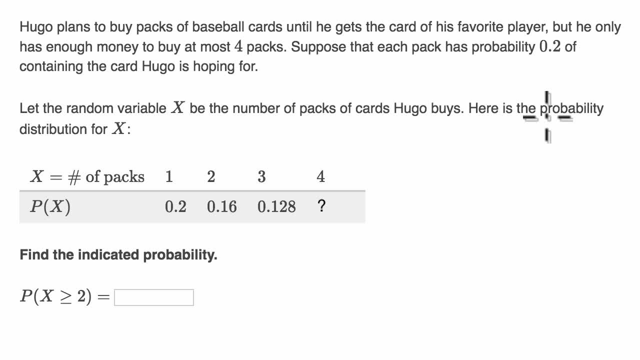 of packs of cards Hugo buys. Here is the probability distribution for x. So it looks like there is a 0.2 probability that he buys one pack and that makes sense because that first pack there is a 0.2 probability that it contains his favorite player's card. 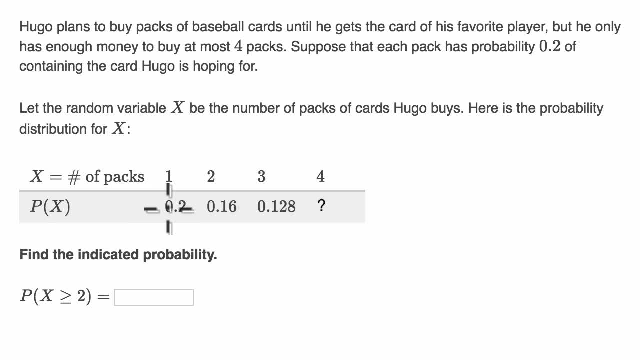 and if it does, at that point he'll just stop. He won't buy any more packs. Now what about the probability that he buys two packs? Well, over here they give it a 0.16, and that makes sense. 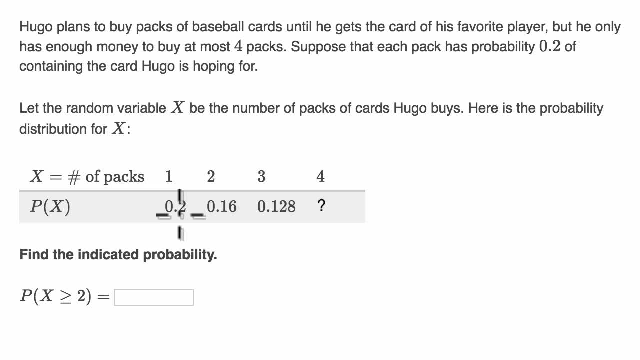 There is a 0.8 probability that he does not get the card he wants on the first one, and then there's another 0.2 that he gets it on the second one. So 0.8 times 0.2 does indeed equal 0.16.. 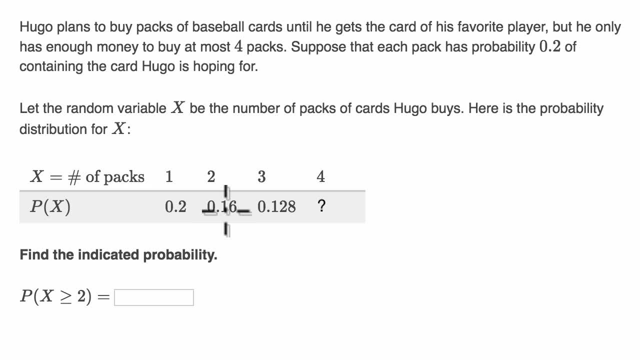 But they're not asking us to calculate that. They give it to us. Then the probability that he gets three packs is 0.128, and then they've left blank the probability that he gets four packs. But this is the entire discrete probability distribution. 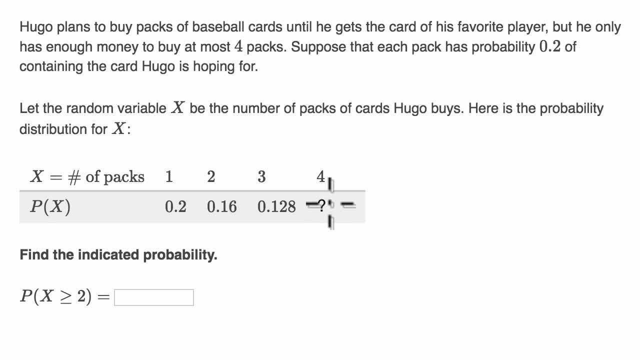 because Hugo has to stop at four. If he doesn't get the card he wants at four on the fourth pack, he's just going to stop over there. So we could actually figure out this question mark by just realizing that these four probabilities have to add up to one. 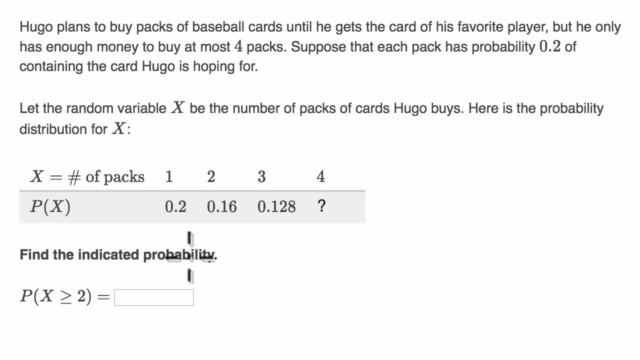 But let's just first answer the question. Find the indicated probability. What is the probability that X is greater than or equal to two? What is the probability? Remember, X is the number of packs of cards Hugo buys. I encourage you to pause the video. 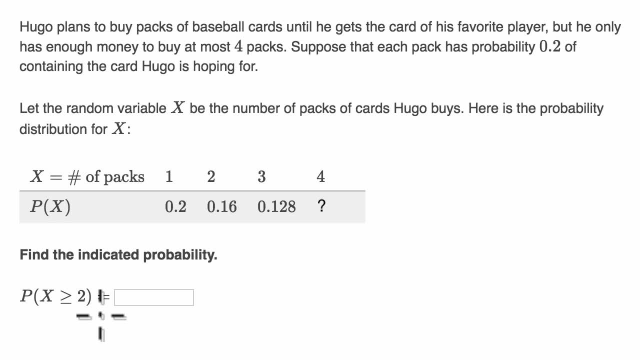 and try to figure it out. So let's look at the scenarios. we're talking about Probability, that our discrete random variable X is greater than or equal to two. Well, that's these three scenarios right over here, And so what is their combined probability?